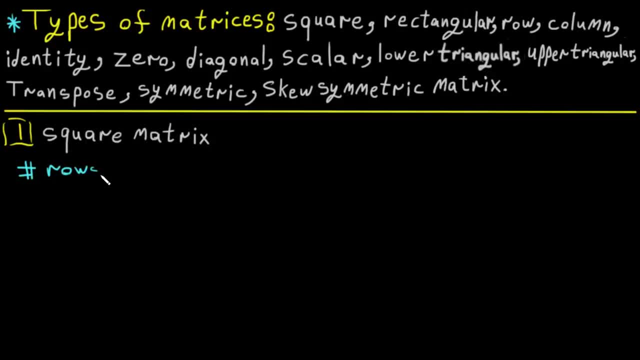 Equal number of column. Here I mean here of this one, number of, I mean of this hash, here number of, and the same as this one. So here number of rows equals number of rows Equal to number of column. for square matrix, For example, the simple one is one by one matrix, For example here minus one, Here one by one matrix, This one. Another example: Five, two, three minus one, This two by two matrix, And so on. We can put here three by three matrix. 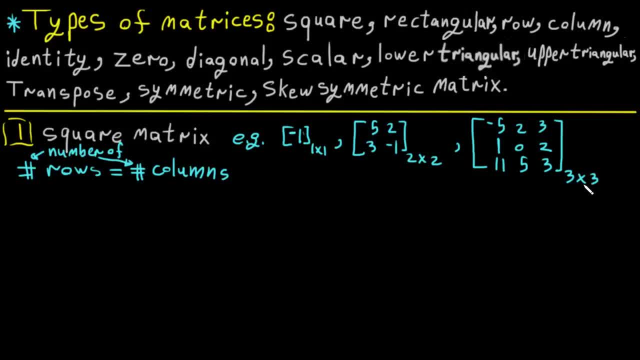 This three by three matrix. I will explain more. what is this one and what is this one? here, This one number of rows, One, Two, And here, in purple, This one Number of columns, The same thing as this one, And of course, here you can put any number of rows. 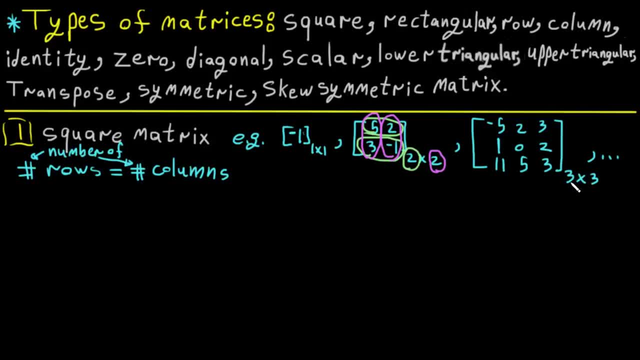 You can put any size as you wish, For example 100 by 100 matrix, which is square matrix. The second one is rectangular. We will write it here Here: rectangular matrix. opposite of this: one number of rows, Not equal number. This I mean number of rows. 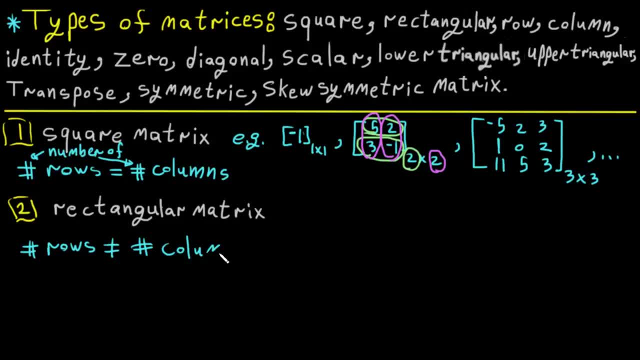 Number of column. For example, This: two by three matrix: Two rows and three column, Which is rectangular matrix. Another example, This one: 4 by 2, and so on. you can write any size you want, of course the number of rows. 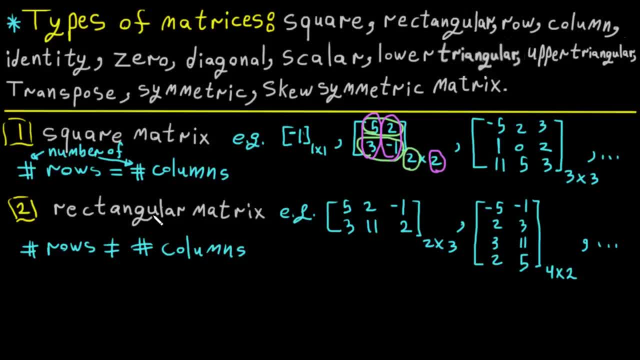 not equal to the number of columns, then it will be rectangular matrix. the third one is row matrix. you row matrix or row Victor, and from here the name row Victor, it's mean only one row. so example of this one, it's very easy, which is like this: one or minus one. 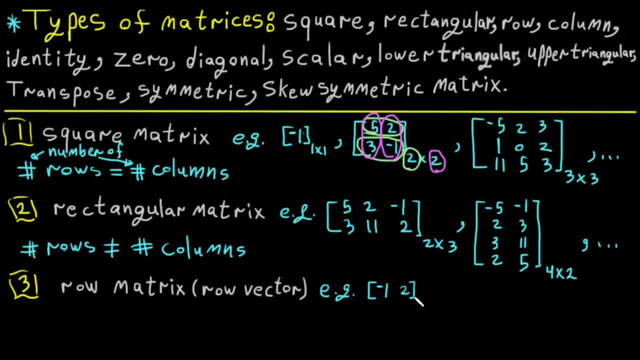 two. it has one row, just one row, one by two. this because one row and two column, and here this one, one by three, and so on, because here three, three column, and, as you noticed, here, here one, here one, so it has only one row. so this is the row. 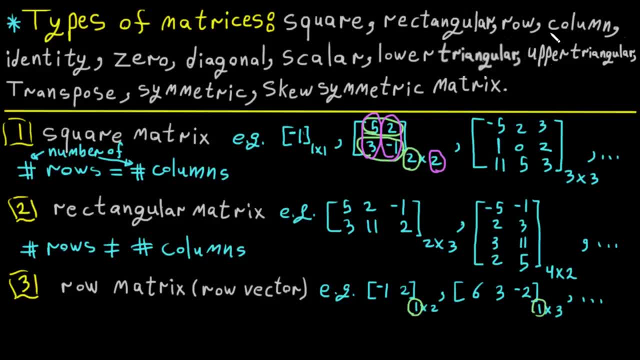 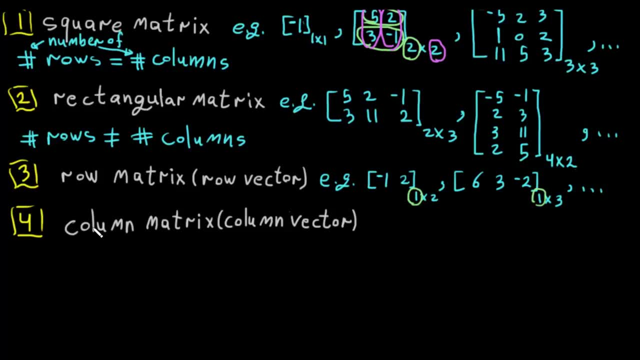 matrix. now we will talk about column matrix. column matrix or column vector, for example. it has only one column. three, two: this has only one column, so this one, two rows and one column, so two by one. another example: this one, three by one, matrix, and so on. as you can see here, it has only one. 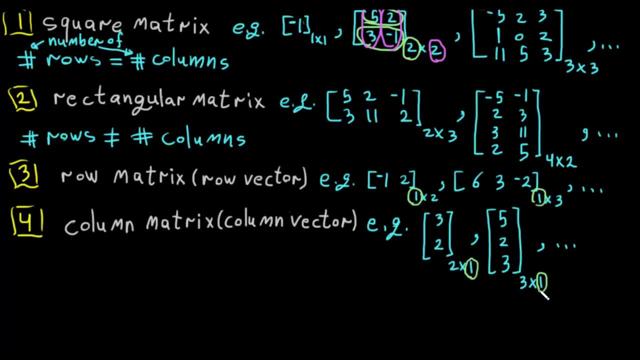 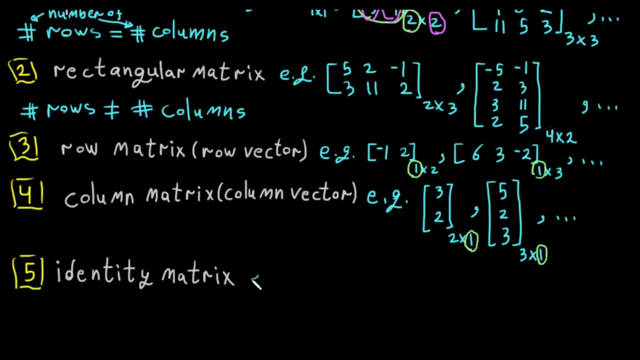 column. this one has only one column. so this is column vectors example for column vector. now we will know about identity matrix. identity matrix, for example, one, this one by one matrix or two by two matrix, one zero, zero one, as you can see here. as you can see here, on the main diagonal, is: 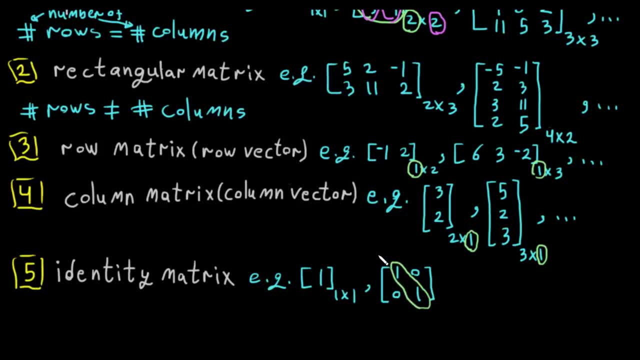 one. here is this called main diagonal. this is main diagonal. here one one, the entries one one and the entries two, two of course. this one two by two matrix, three by three matrix, and here an identity matrix has ones on the main diagonals and everywhere else are zeros, so here zero. 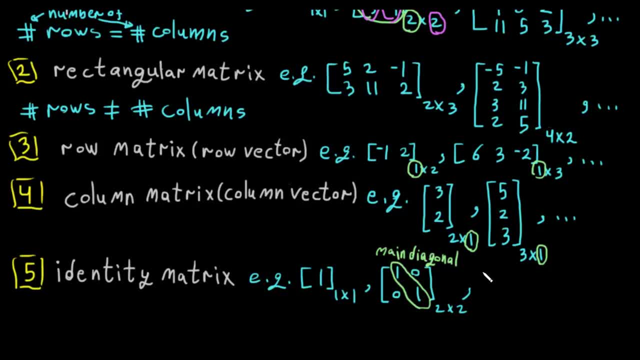 Let's introduce three by three matrix, this as three by three matrix, as you can see that there is one in this column, here or on here on the main diagonal, and notes. think of this as three by three matrix, As you can see here. here you can see there are onlyikoamas here on the main diagonal, and everywhere else are zeros, or zeroes. here, that is known, by the way, and all the 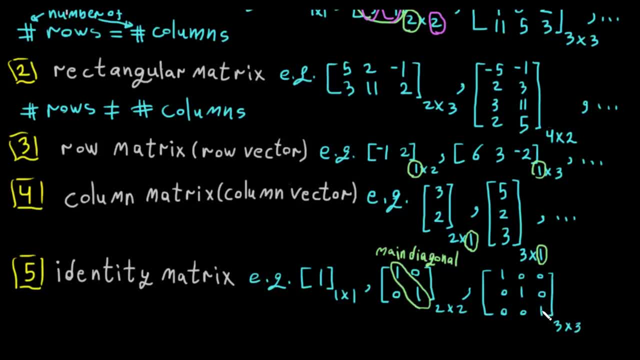 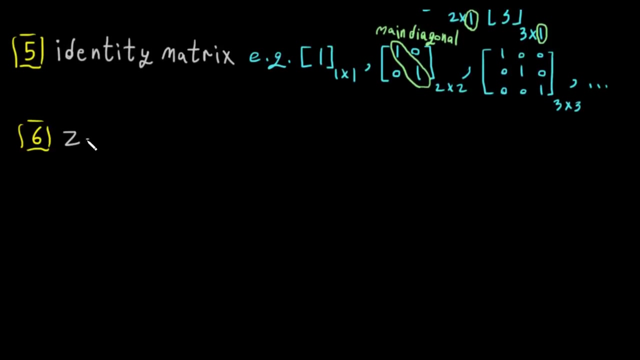 order of here, on the main diagonal ones and everywhere else are zeros, and so on. you can put 10 by 10 matrix which has the same thing on the main diagonal ones and everywhere else are zeros. now we will introduce the zero matrix. you here's your matrix, or they called it null matrix, which is very simple. 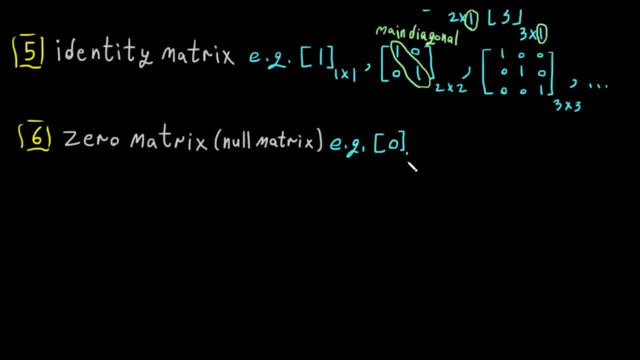 Zero, here only zero. this is one by one matrix, its opposite of this. one, here only one and here only zero. or you can write zero, zero, zero, zero, this two by two matrix, and they called it null matrix or zero matrix. you can put two by three, three by two, three by three or any size you wish. now we will. 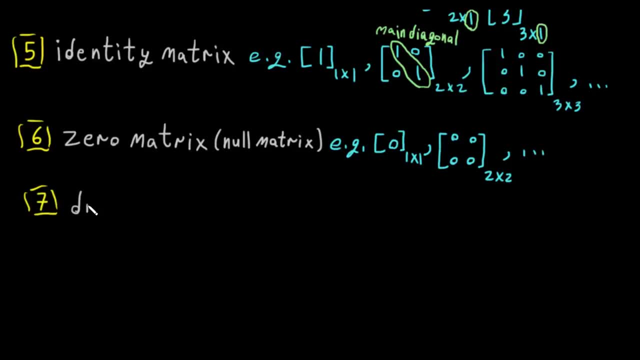 talk about diagonal matrix, diagonal matrix, diagonal matrix. it's similar to identity matrix, but in diagonal matrix has numbers here not equal to zero. so for example, here two zero, zero minus one. you can see here on the main diagonal numbers and everywhere else are zero. so a diagonal. 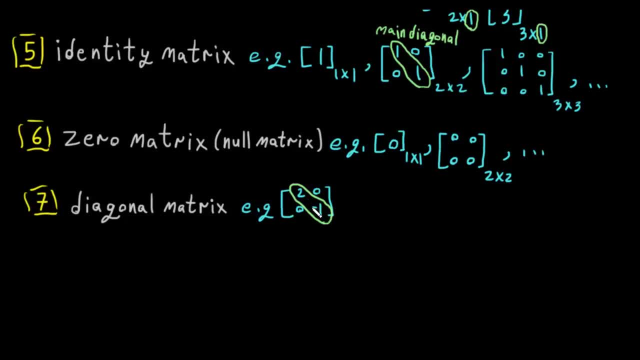 matrix has 0 everywhere except the main diagonal. this 2 by 2 matrix- let's put example for 3 by 3 matrix, as you can see here on the main diagonal here has number. everywhere else are 0. this is 3 by 3 matrix, and so on. now we'll introduce the scalar matrix. 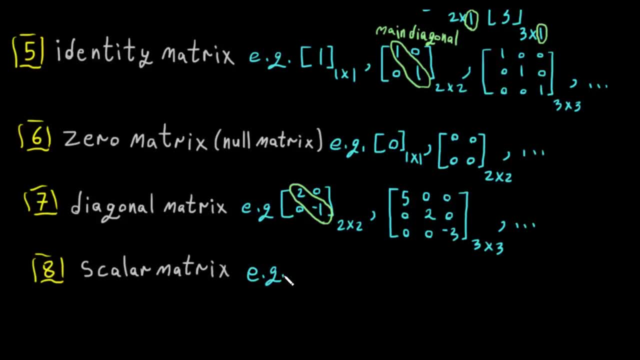 example of scalar matrix. scalar matrix has similar to identity matrix, but here in scalar matrix has numbers on the main diagonal and they are the same. so a scalar matrix has all main diagonal entries the same with 0 everywhere else. so here 0 and here the same numbers. this is 2 by 2. 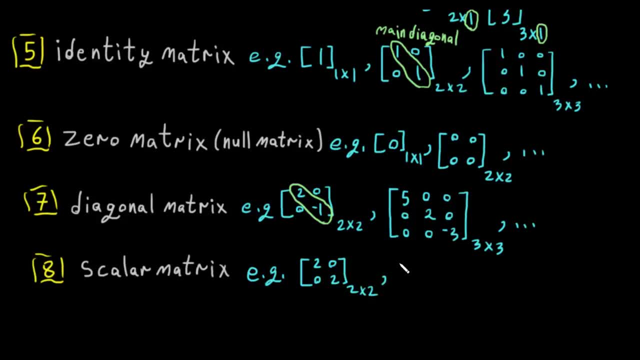 matrix. another example: 3, 0, 0, 3. this is scalar matrix because they have the same number. add everywhere else are 0. this is the same 2x2 matrix. for 3x3 matrix we will put example here: 3x3 matrix. 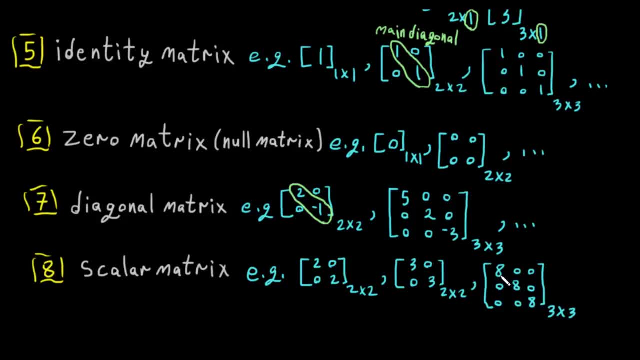 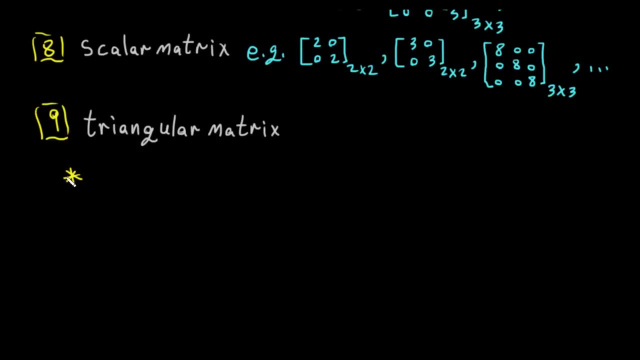 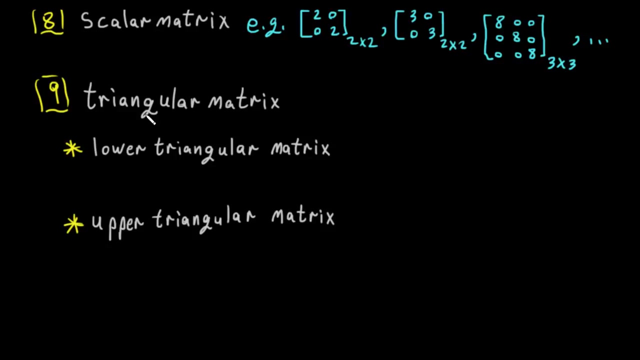 so the main diagonal here has the same number, 888. so this is scalar matrix and so on. now we will introduce triangular matrix. here we have triangular matrix and here triangular matrix has either lower triangular matrix or upper triangular matrix. you can say: this one is triangular matrix. but if you want to be more specific you can say: 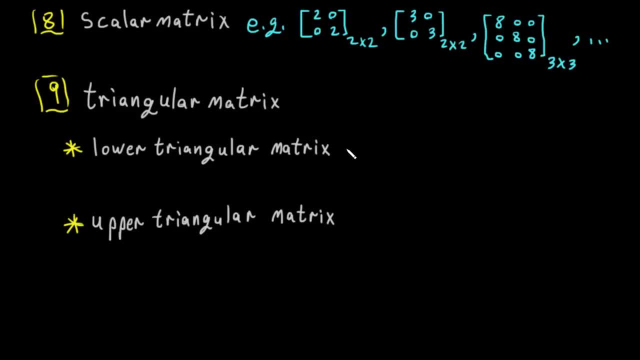 lower triangular matrix or upper triangular matrix. what is lower triangular matrix, for example? let's look like this, for example here: 5,, 0,, 3, minus 2, this is 2x2 lower triangular. why it's triangular matrix? because here we have right triangle. 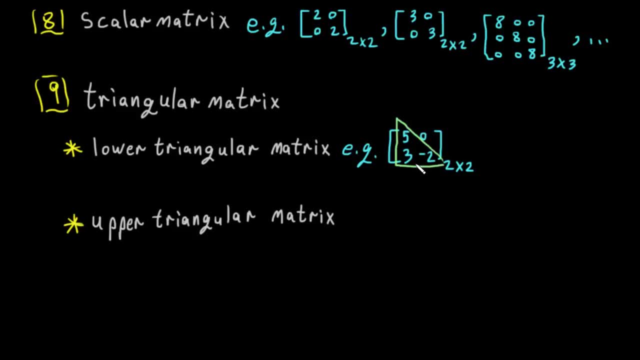 you can see, here we have right triangle and here, if this shape like this, then it is lower triangular matrix. another example for 3x3 matrix: this is 3x3 matrix and, as you can see here, right triangle. look like this here and so on. 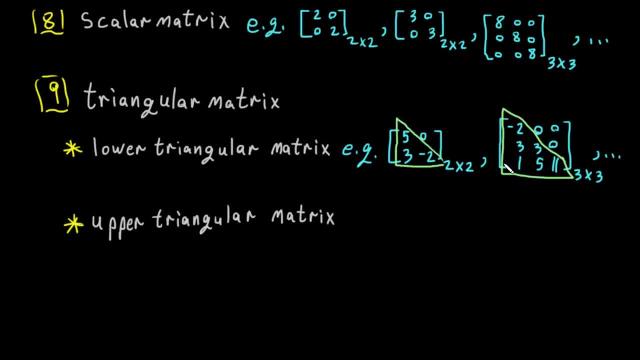 this is lower triangular matrix, as you can see here. the right angle here, right angle here for upper triangular matrix. this angle, it's opposite. it will be here. for example, here let's look like this: 2, 5, 0, minus 3x2. 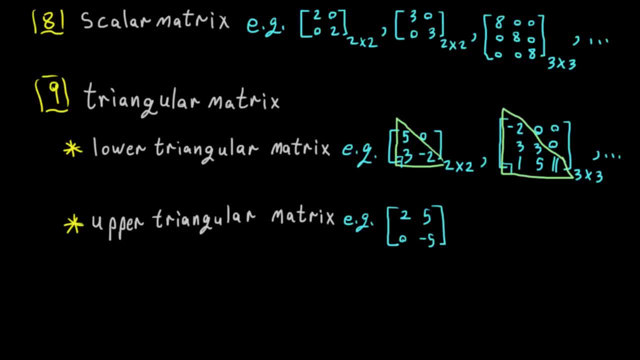 5, for example. see right triangle, look like this. and here the right angle here. so that's why this called upper triangular matrix. another example: 3x3 matrix. the right triangle is like this, the right triangle here here. it has here 90 degree, and so on. 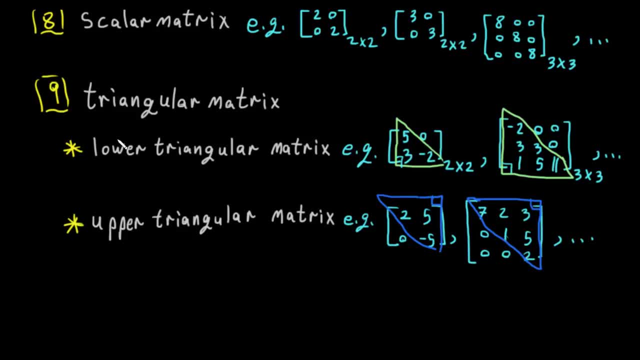 lower triangular matrix is when all entries above the main diagonal 0, above the main diagonal 0. where upper triangular matrix is when the all entries below the main diagonal 0 is when the all entries below the main diagonal 0. main diagonal is 0. so here below the main diagonal are zeros. now we will. 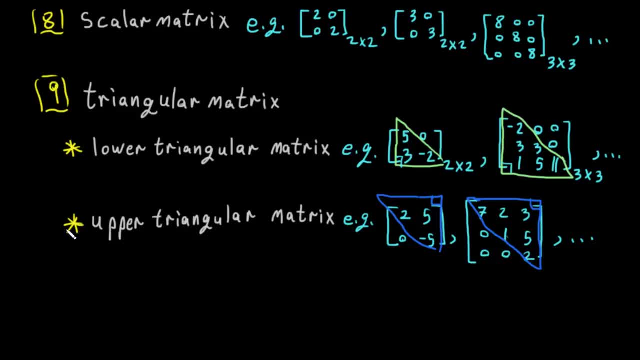 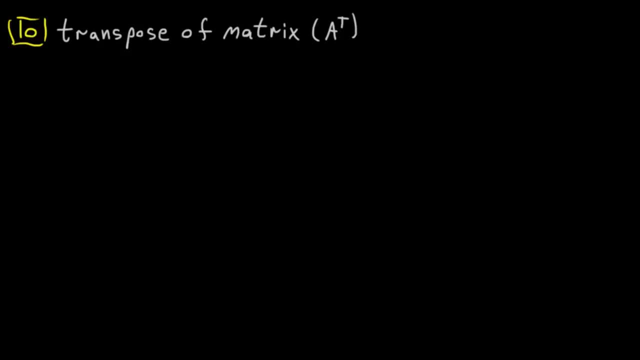 introduce for you transpose of matrix. transpose of matrix is very simple. it's only you have to swap the rows and column, so rows become columns and columns become rows. it's very simple. here, for example: let's we have a equal, so here the a transpose the symbol of transpose. here it's look like this: so a. 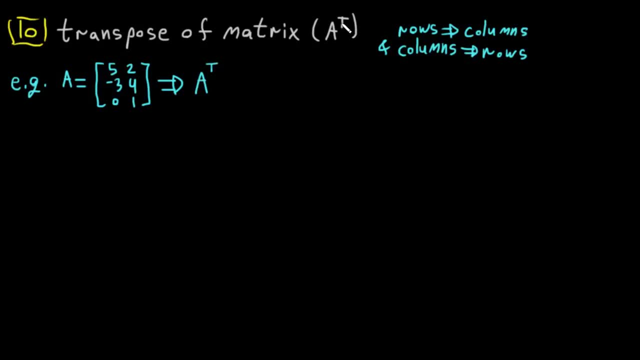 transpose. this is transpose, here T equal. we have to swap the rows with column. so here, this row, it will become column, so five. two: I swap this one to here the same thing. here this row, it will become column, so negative three. four: this row become column, so zero one. 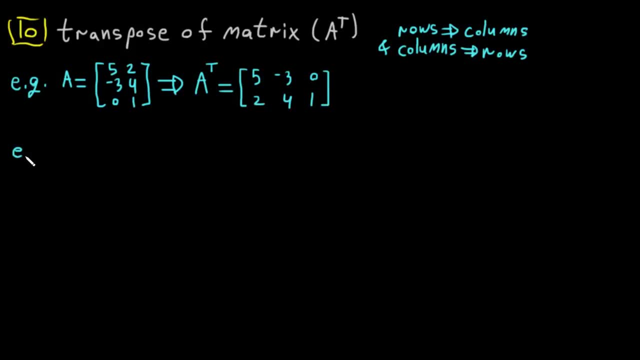 another example be equal. I'll put symbol example here: five, two, nine, five, two, nine, five, two, nine 就是 this: one by three, because one row by three, columns b, transpose: BeTrahsalle is the Draw With The New. Huh, we have to swap this row to become column, so it will be like this: 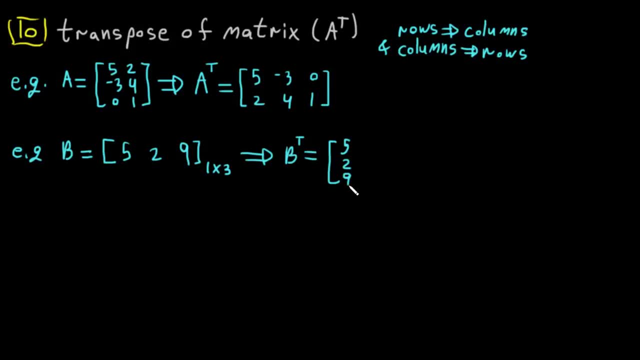 to be irresponsible. So what we're doing- truss all your tables, if I items and how to transform them- is to calculate what the unit column and column parts would be times to be added. to determine which column it would be, three by one the same. here we have three rows and two column. three rows, two column, then after. 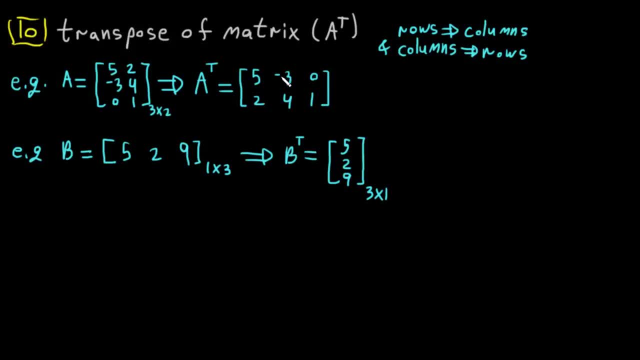 the transpose, this one transformed to 2 by 3, so a 3 by 2. transform to this matrix which is 2 by 3, so a transpose 2 by 3. now we will talk about the negative of matrix here. it's very simple: the negative of matrix, for example, if we have, let's say, 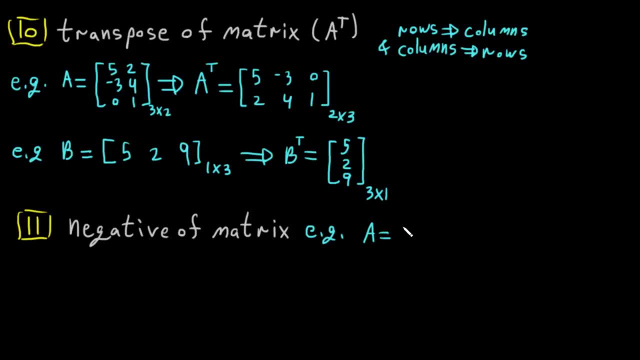 a equal 5, 5, 2, 0 minus 3, then the negative of a, the negative of matrix, a equal. we have only to multiply 5. multiply by negative 1, which is minus 5, multiply by negative 1, which is minus 2. this one, it's. 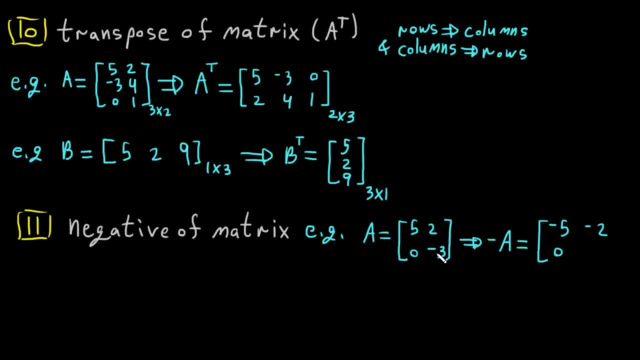 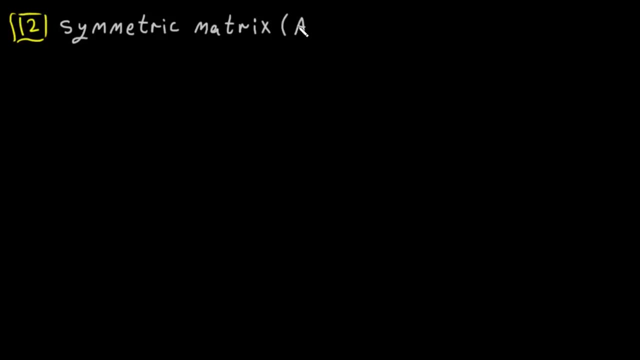 it we will remain the same. minus 1, multiplied by minus 3, it will be 3. now we will know about symmetric matrix. here we have symmetric matrix, which is a equal a transpose. so if this condition satisfy, then we can say symmetric matrix, so a matrix whose transpose is the same as the ordinal. 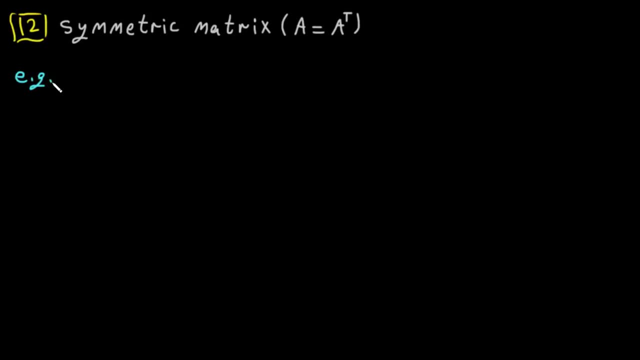 matrix, for example a, this is given matrix. so if we want to test if this symmetric or not, we have to take the transpose. so let's write it in another color. so then a transpose equal. so this one. it will become column one, two, three. this row will become the. 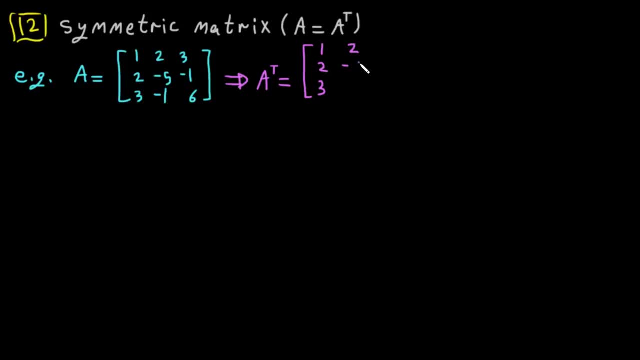 column two minus five minus one. this row, the third row, it will be the third column. so three negative one, six. let's compare these two. so one, one, two, two, three, three, two two negative five negative, five negative one negative one. three, three minus one minus one six, six. 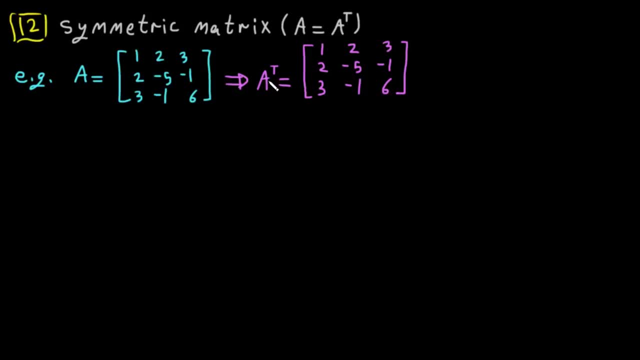 since these matrices are equal, then, or since a a equal a transpose, then a is symmetric matrix. now we'll introduce for you the skew symmetric matrix. here we have skew symmetric matrix. it is skew symmetric matrix if satisfy this condition: a transpose equal to the negative of a. this mean a matrix whose 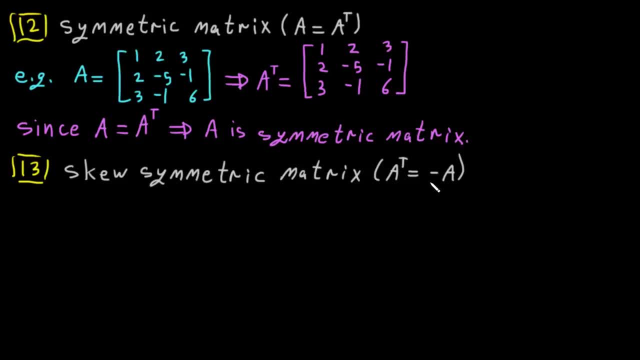 transpose is equal to the negative of the ordinal matrix. example for this one, let's use this test a transpose, throwing a AE and putting it on the interessante. so vale to campus. lets say this: a will be that to test the skew symmetry. let's say we have this a. 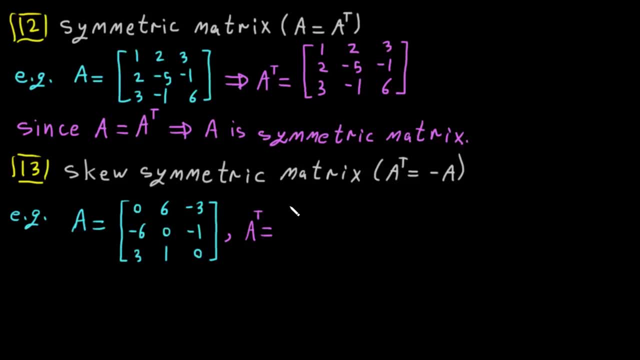 to test if this skew symmetric or not, they have to compute a transposes with the negative of a. so here we will compute this one first: a transpose row to become column zero six negative three, and this row to become column negative six: zero negative one. the last row, it will become the last column here.